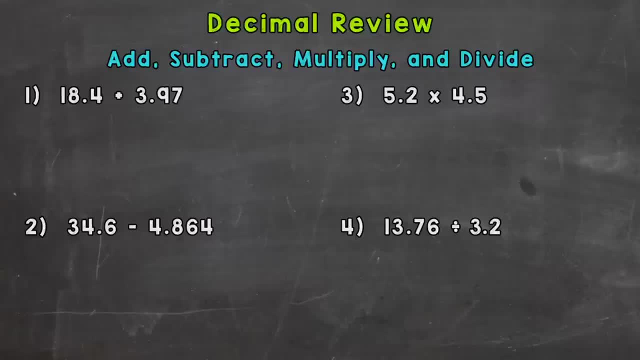 multiplying, and dividing decimals below in the description. So let's jump right into number one here where we have addition. So 18 and 4 tenths plus 3 and 97 hundredths. So for adding and subtracting decimals the most important part is lining the problem up correctly. 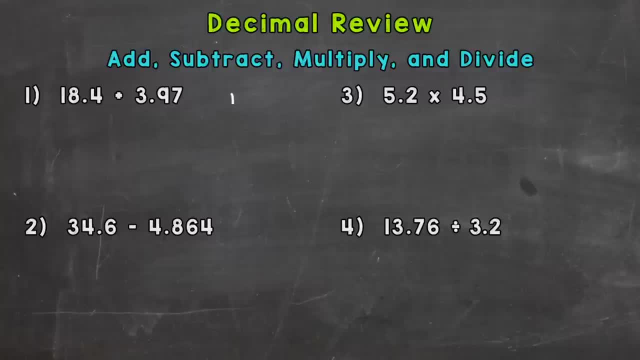 And you do that by lining up your decimals. So 18 and 4 tenths plus 3 and 97 hundredths. Now the problem looks a little offset. That's fine. We can use placeholder zeros because zeros to the right of a decimal do not change the value. So I can put a zero here to the right of that. 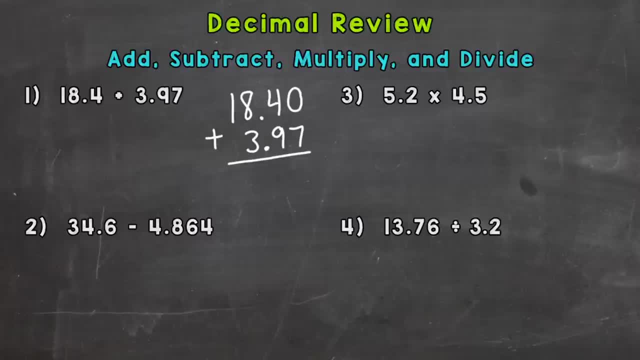 And it doesn't change the value. It's an equivalent decimal. So now it looks a little neater and more lined up. So once you have your decimals lined up and any placeholder zeros put into place we can just add. So 0 plus 7 is 7. 4 plus 9 is 13. Bring my 1 over here. Now decimals line up throughout the whole problem. 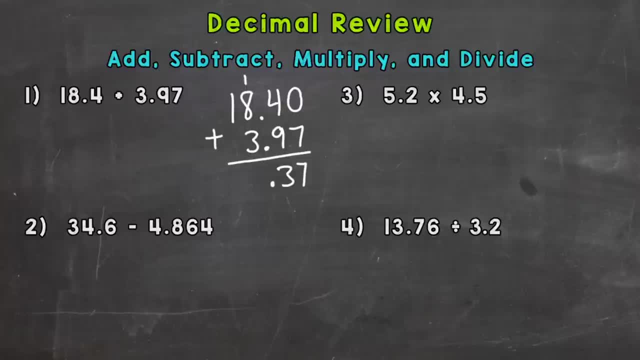 So bring it straight down. 1 plus 8 is 9 plus 3 is 12. 1 plus 1 is 2. So our answer is 22 and 37 hundredths. 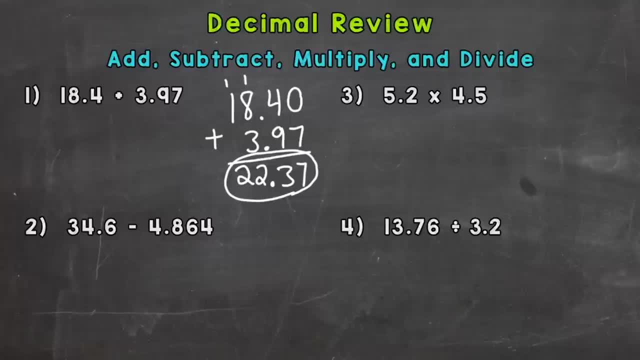 Now let's take a look at our original problem. With decimals it's good to always see if your answer makes sense and we can use estimation. So this number 18 and 4 tenths is around 18. And the second number, 3 and 97 hundredths, if we were to round that to the nearest whole, it would be around 4. So 22 is a good estimate. So our answer, 22 and 37 hundredths, is a 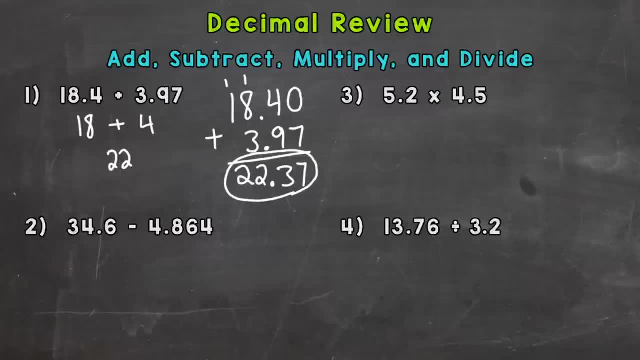 reasonable answer. If you put the decimal in the wrong place or forgot the decimal, it should tell you that something went wrong because that answer doesn't make sense. So let's take a look at number 2. 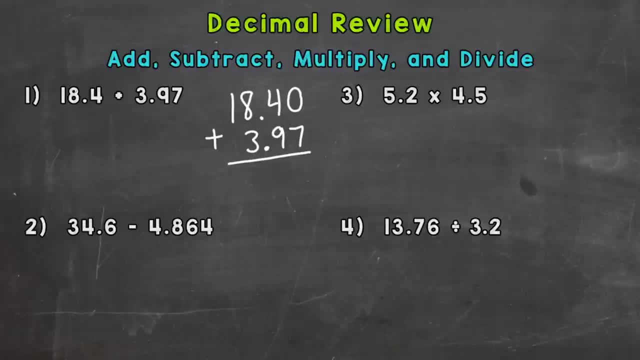 we can just add. So 0 plus 7 is 7.. 4 plus 9 is 13.. Bring my 1 over here Now. decimals line up throughout the whole problem. So bring it straight down: 1 plus 8 is 9 plus 3 is 12.. 1 plus 1 is 2.. So our answer is 22 and 37 hundredths. 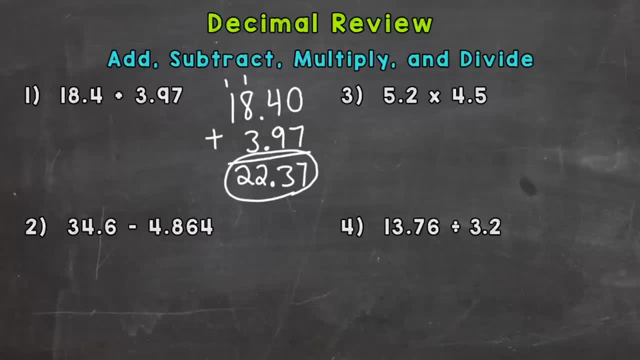 Now let's take a look at our original problem With decimals. it's good to always see if your answer makes sense and we can use estimation. So this number, 18 and 4 tenths, is around 18.. And the second number, 3 and 97 hundredths, if we were to round that to the nearest whole. 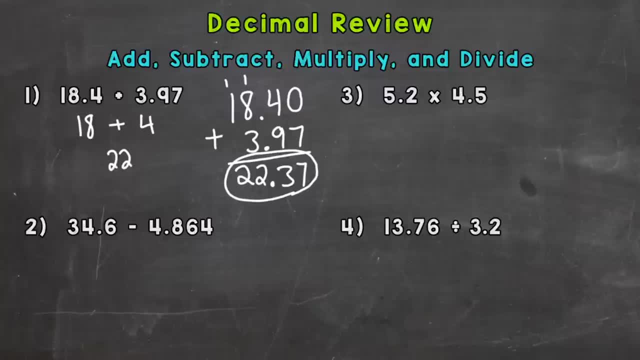 it would be around 4.. So 22 is a good estimate. So our answer- 22 and 37 hundredths- is a reasonable answer. If you put the decimal in the wrong place or forgot the decimal, it should tell you that something went wrong, because that answer doesn't make sense. So 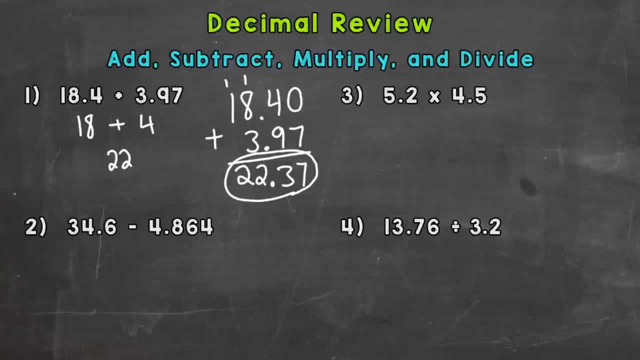 let's take a look at number 2. Again, adding and subtracting. the most important thing: line your decimals up. So here we have 34 and 6 tenths minus 4 and 864 thousandths. Now that problem looks even more. 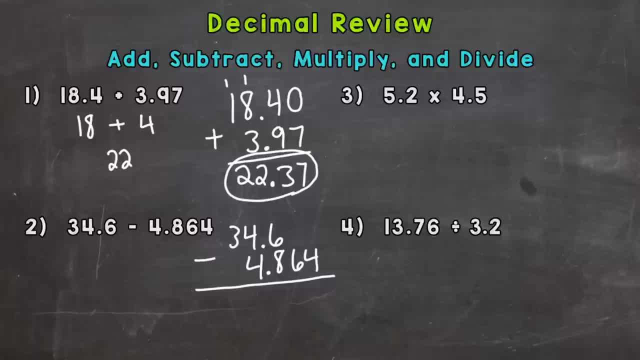 offset than the first one. That's okay, because we lined our decimals up, the most important part, And when you line your decimals up, it lines all of your problems. So now we need a couple of placeholder zeros. Now we're all lined up and we have our placeholder. 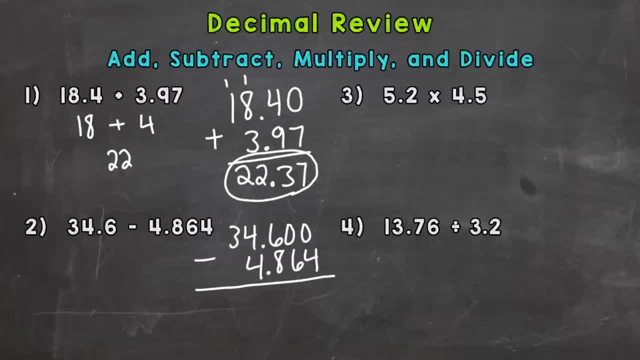 zeros. I cannot do 0 minus 4.. I need to borrow. So I can't borrow from this 0, so I need to borrow from the 6.. It's now a 5.. This 0 turns to a 10, but I need to bring the 1 over all. 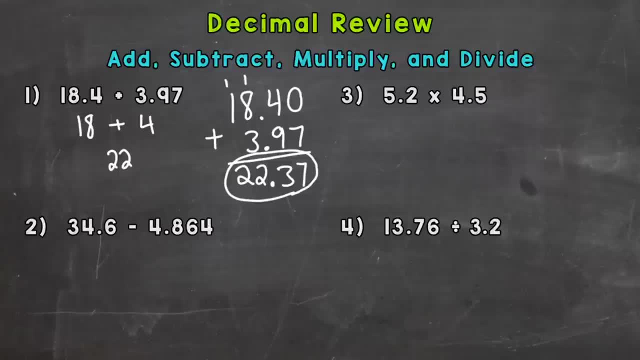 Again adding and subtracting the most important thing, line your decimals up. So here we have 34 and 6 tenths minus 4 and 864 thousandths. Now that problem looks even more offset than the first one. That's okay because we lined our decimals up, the most important part. And when you line your decimals up, it lines your places up. So now we need a couple of placeholder zeros. Now we're all lined up and we have our placeholder zeros. I cannot do 0 minus 4. I need to borrow. So I can't borrow from this 0, so I need to borrow from the 6. It's now a 5. This 0 turns to a 10, but I need to bring the 1 over all the way to the right. So it's going to be a 10. It's going to be a 9. And then the 0 to the far right is now a 10. So 10 minus 4 is 6. 9 minus 6 is 3. 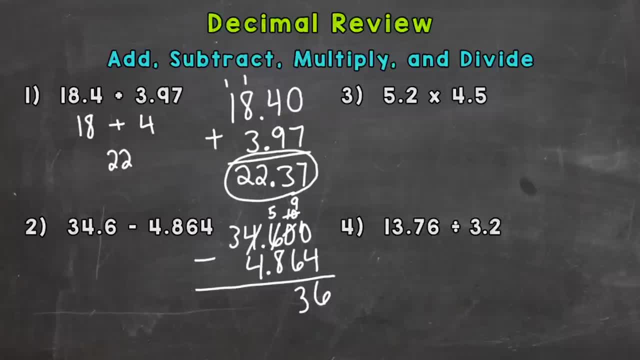 I cannot do 5 minus 8, so I need to borrow from the 4, which now becomes a 3. So I get 15 minus 8, which is 7. Bring my decimals straight down. I need to borrow again from the 3, which is now a 2. And that other 3 now becomes a 13. 13 minus 4 is 9. And then bring my 2 down. 2 minus 0 there would give me 2. 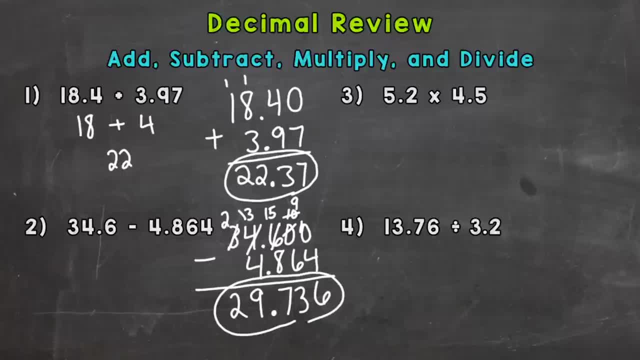 So 29 and 736 thousandths. So let's estimate here. Let's do an estimation. So 34 and 6 tenths would round to 35. 4 and 864 thousandths would round to 5. So 35 minus 5, our estimation would be 30. So our actual answer is reasonable. It makes sense. 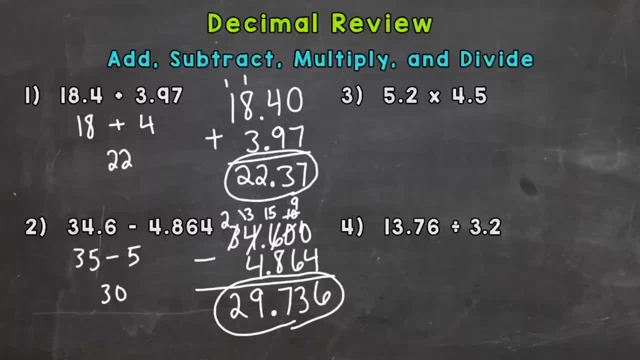 Let's check number 3 as we move to multiplication. So for multiplication, you don't necessarily have to line that decimal up. I find it easier. Let's take out the decimals to start with. And we are going to do 52 times 5. 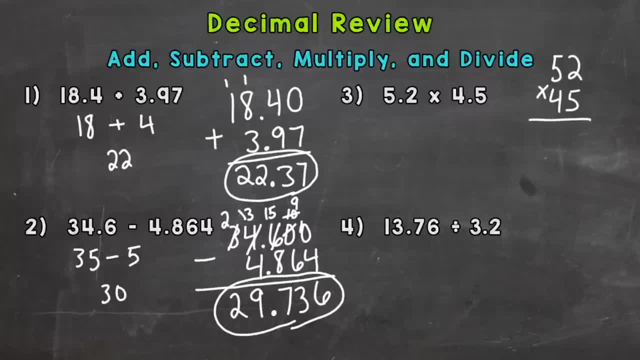 Times 45. Again, I took out the decimals. I'm going to put them in at the end. 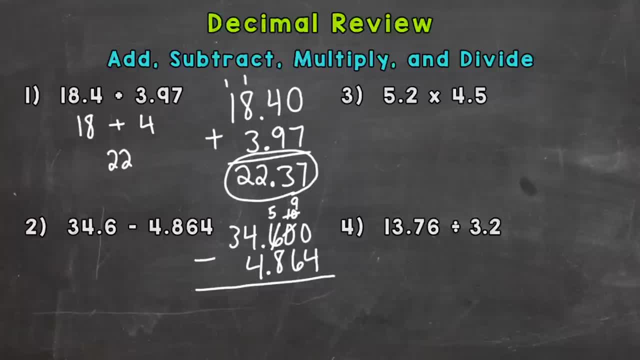 the way to the right. So it's going to be a 9, and then the 0 to the far right is now a 10.. So 10 minus 4 is 6.. 9 minus 6 is 3.. I cannot do 5 minus 8,, so I need to borrow from the 4, which now. 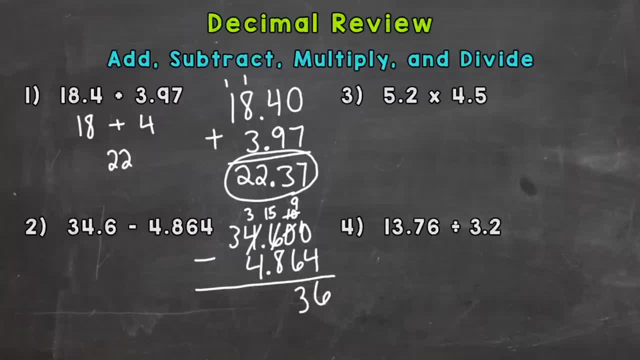 becomes a 3.. So I get 15 minus 8, which is 7.. Bring my decimal straight down. I need to borrow again from the 3,, which is now a 2.. This is the 1 that관 pleasure number, The under Kyle's. 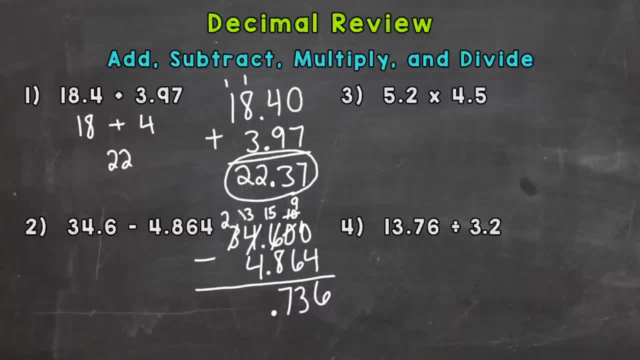 and that other 3 now becomes a 13.. 13 minus 4 is 9.. And then bring my 2 down: 2 minus 0 there would give me 2.. So 29 and 736 thousandths. So let's estimate here, Let's do an estimation. 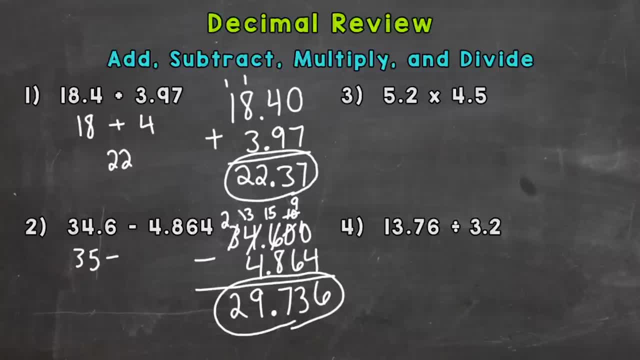 So 34 and 6 tenths would round to 35.. 4 and 864 thousandths would round to 5.. So 35 minus 5, our estimation would be 30.. So our actual answer is reasonable. It makes sense. 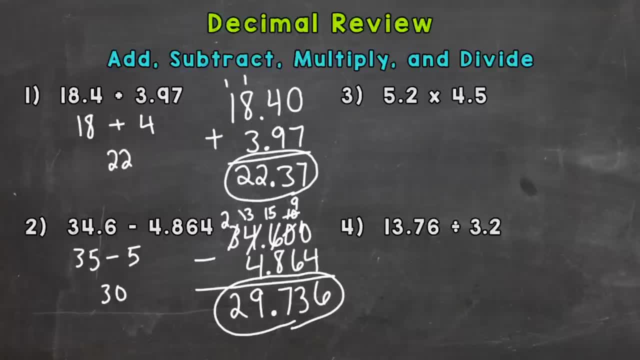 Let's check number 3 as we move to multiplication. So for multiplication you don't necessarily have to line that decimal up. I find it easier. Let's take out the decimals to start with, And we are going to do 52 times. 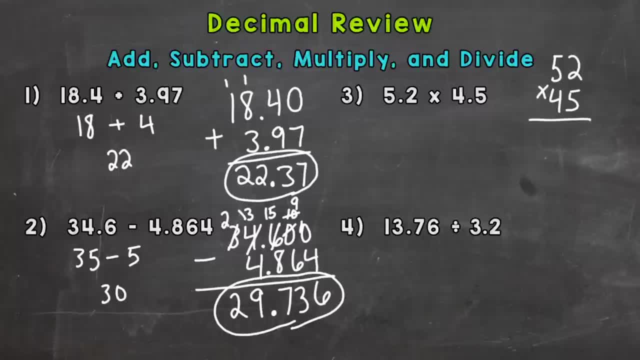 45. Again, I took out the decimals. I'm going to put them in at the end: 5 times 2 is 10.. 5 times 5 is 25.. Plus 1, 26.. Done here. Done here. 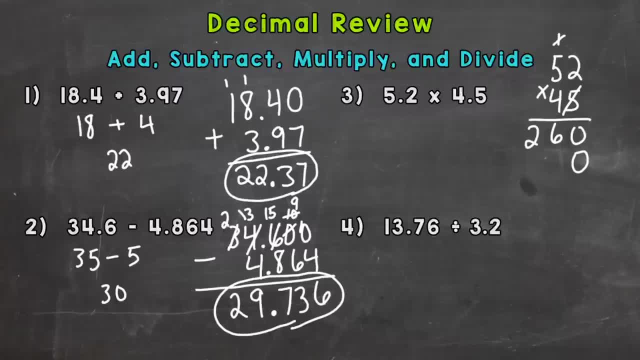 We need our 0 here as we move to the next place. 4 times 2 is 8.. 4 times 5 is 20.. 4 times 5 is 20.. Now we add our partial products: 0 plus 0, 0.. 6 plus 8 is 14.. 1 plus 2 is 3.. And we have our 2 here. 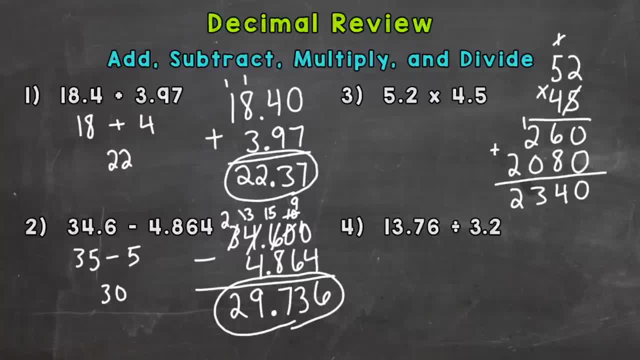 Now we need to put our decimal back in to our answer. So we take a look back at our original problem And we need to see how many digits are to the right or behind a decimal. Well, we have this 2 here, So that's 1.. 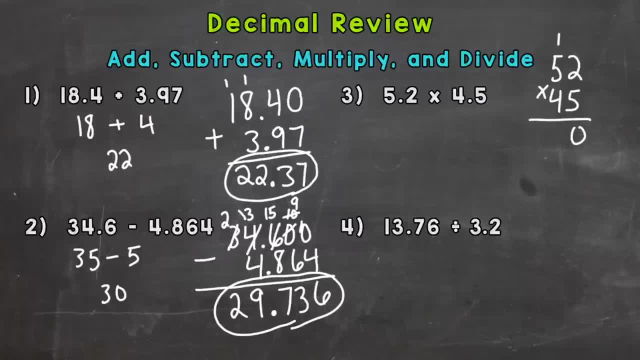 5 times 2 is 10. 5 times 5 is 25. Plus 1, 26. Done here, done here. We need our 0 here as we move to the next place. 4 times 2 is 8. 4 times 5 is 20. Now we add 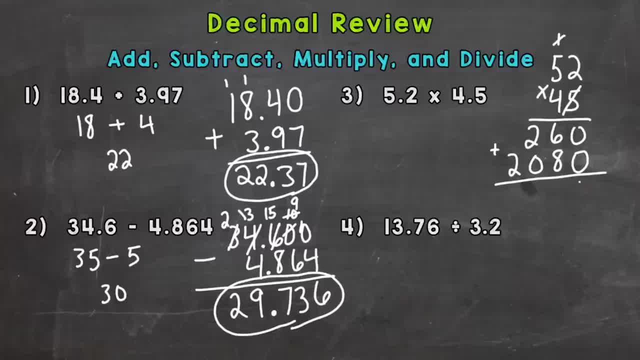 our partial products. 0 plus 0 is 0. 6 plus 8 is 14. 1 plus 2 is 3. We have our 2 here. 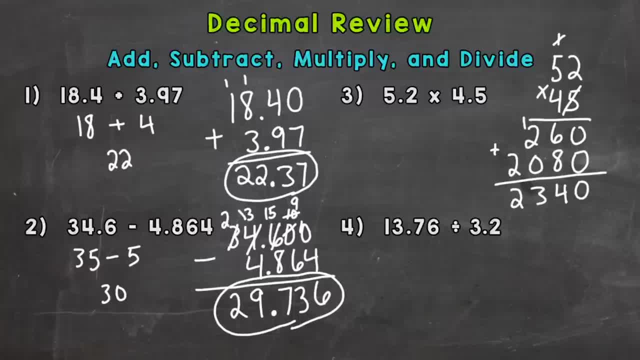 Now, we need to put our decimal back up to our answer. So we take a look back at the original problem, a we need to see how many digits are to my turn We need to see how many digits are to the right or behind the decimal. We get this 2 here, so that's 15. Now, let's divide these by count. Well, we have this 2 here, so that's 1. And we have this 5 here, so that is 2. Two digits behind the decimal, so our answer needs two digits behind the decimal. So we bring it in, 1, 2. 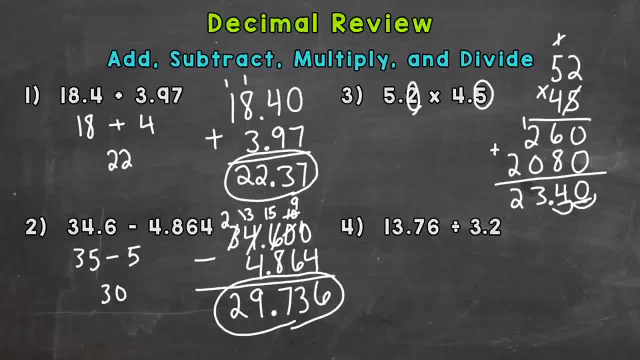 And it goes right here, or think of it as 1, 2 digits behind the decimal in our answer. 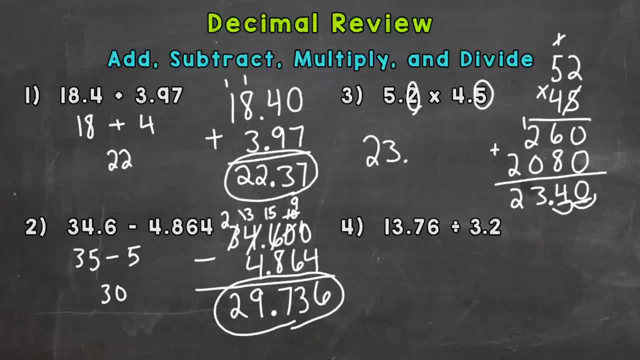 So for number 3, the product is 23 and 40 hundredths. And if we take a look at our original problem, we have something around 5 times something around 5. So our answer should be somewhere around 25. So our answer is reasonable. We know we put the decimal in the correct place. 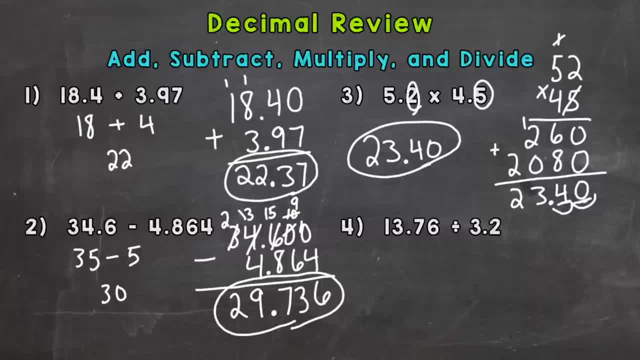 So for number 4, we have dividing decimals. So let's set it up. 3 and 2. 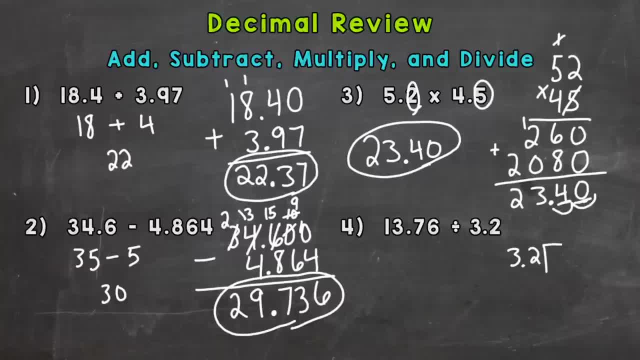 2 tenths is our divisor. And 13 and 76 hundredths is our dividend. So when you get to division problems, the first thing we need to check is, is the divisor, or outside number, whole? If not, we need to make it a whole number. Here we have 3 and 2 tenths, so it's not exactly a whole. So we need to move this decimal to the right. One time, to make it a whole number. This is going to make our problem much easier. Now, whatever you do to the outside, you have to do to the inside. 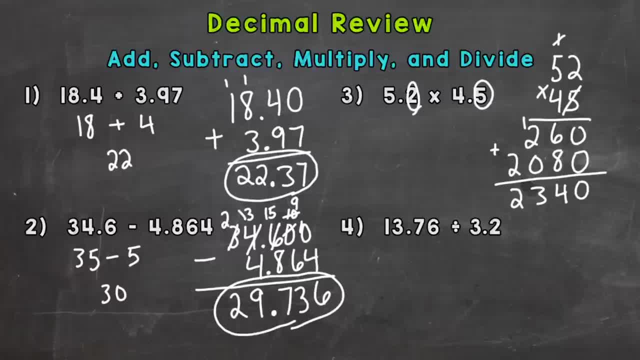 And we have this 5 here. So that is 2.. Two digits behind the decimal. So our answer needs two digits behind the decimal. So we bring it in 1, 2. And it goes right here. Or think of it as: 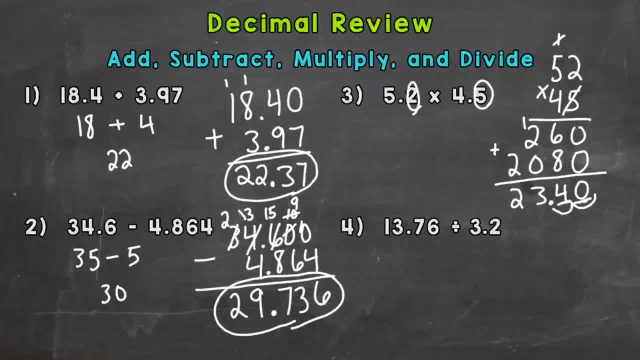 1, 2 digits behind the decimal in our answer. So for number 3, the product is 23 and 40 hundredths And if we take a look at our original problem, we have something around 5 times, something around 5. So our answer should be somewhere around 25.. So our answer is reasonable. We. 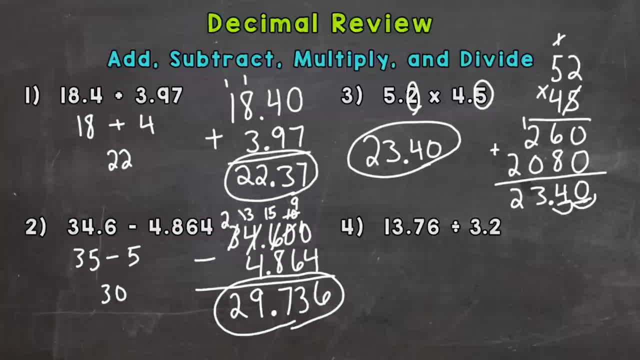 know we put the decimal in the correct place. So for number 4, we have dividing decimals, So let's set it up: 3 and 2 tenths is our divisor And 13 and 76 is our divisor, So we have the divisor And 13 and 76 is our dividend. So when you get to division problems, 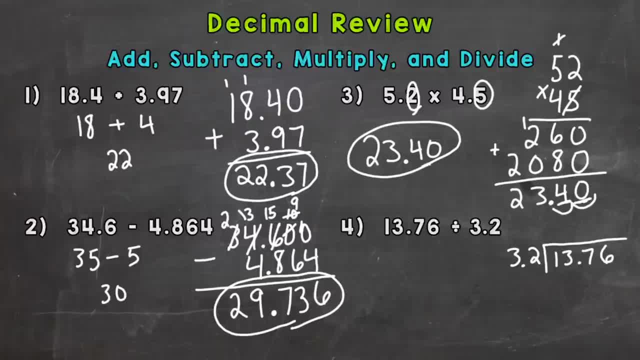 the first thing we need to check is: is the divisor or outside number whole? If not, we need to make it a whole number. Here we have 3 and 2 tenths, So it's not exactly a whole. So we need to move this decimal to the right one time to make it a whole number. This is 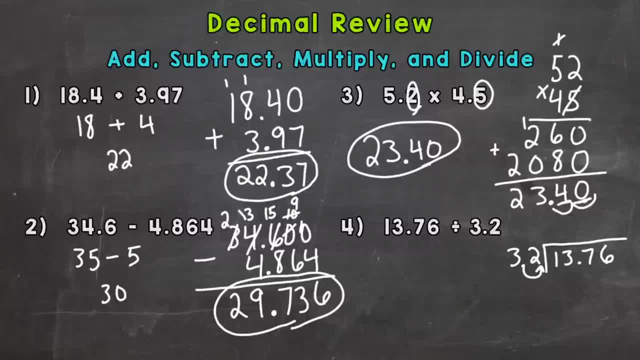 going to make our problem much easier. Now, whatever you do to the outside, you have to do to the inside. Everything needs to stay balanced. So we moved it once to the right on the outside. So we need to move it once to the right on the inside. Now we can rewrite our problem. So. 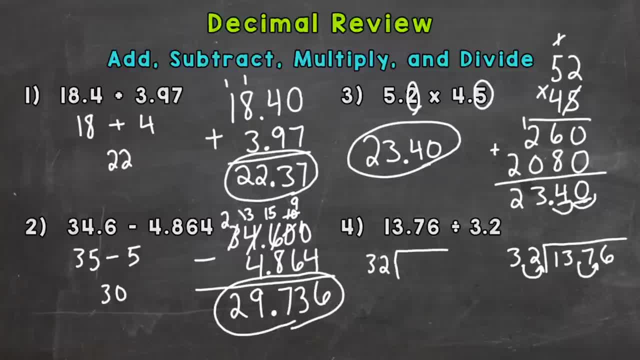 we have 32 as our divisor And we have 137 and 6 tenths. Now that the divisor is whole, we bring this decimal straight up. That's the decimal that we're going to use And we're going to place it in the answer. That's where it's going to be placed in the answer. So if you 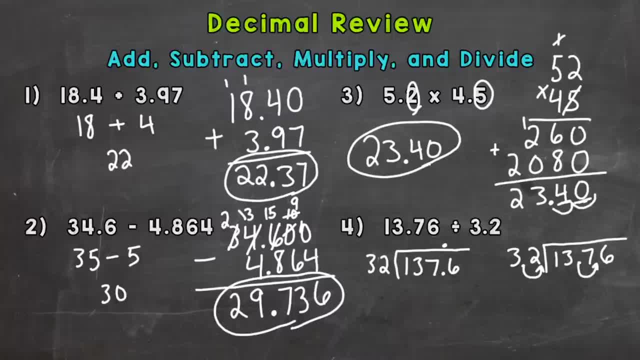 have a whole number on the outside, right off the bat. you can bring that decimal straight up right away. But here, in this case, we did not. So now we can go through our long division steps. Can we do 1 divided by 32? No. Can we do 13 divided by 32? No. So we 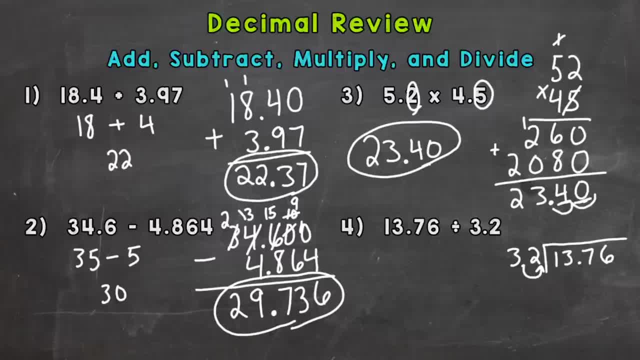 Everything needs to stay balanced. So we moved it once to the right on the outside. So we need to move it once to the right on the inside. 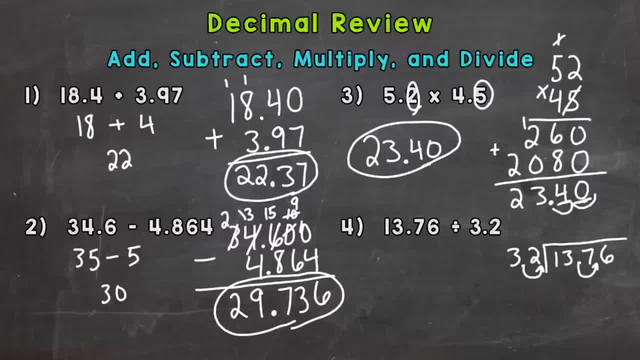 Now we can rewrite our problem. So we have 32 as our divisor. And we have 132. And we have 132. And we have 37. And 6 tenths. 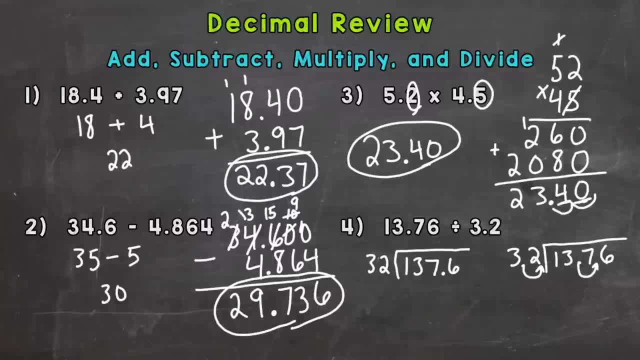 Now that the divisor is whole, we bring this decimal straight up. That's where it's going to be placed in the answer. 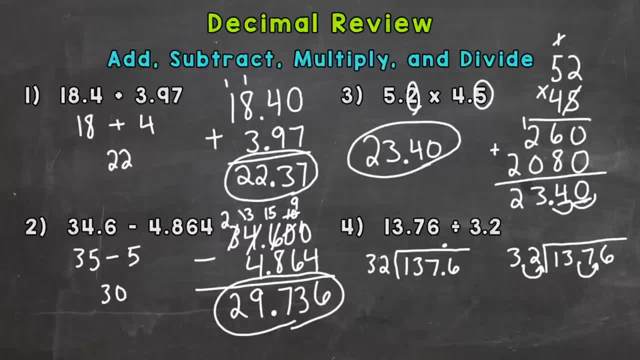 So if you have a whole number on the outside, right off the bat, you can bring that decimal straight up right away. But here, in this case, we did not. So now we can go through our long division steps. 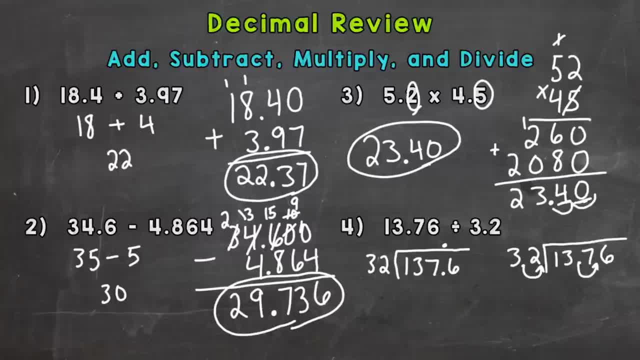 Can we do 1 divided by 32? No. Can we do 13 divided by 32? No. Can we do 3 divided by 2. 3, I'm sorry, 13 divided by 32. No. 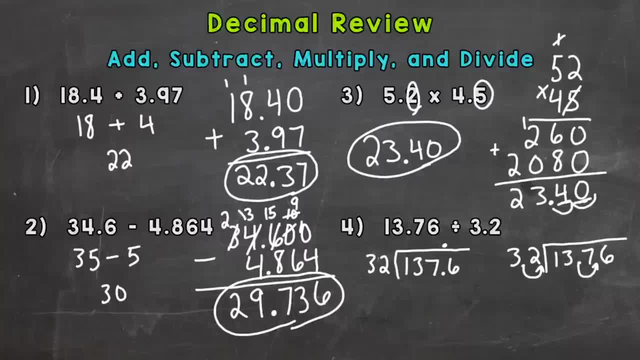 So we need to do 137 divided by 32. And 32 can be pulled out of 137 four times. 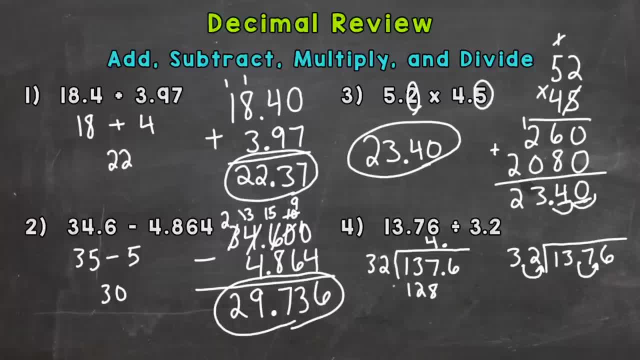 That gets us to 128. So we'll subtract. We get 9. Bring down this 6. 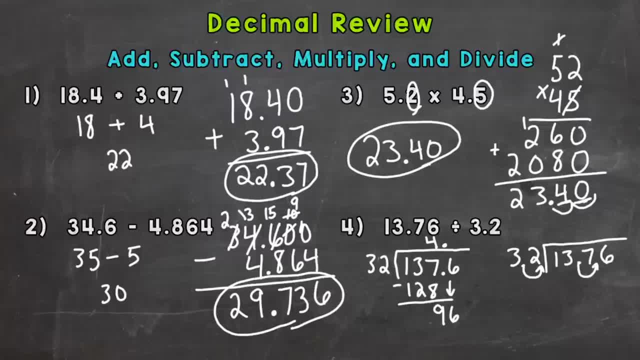 So now we have 96 divided by 32, which happens to be 37. which happens to give us three. We can pull three whole 32s out of 96, and 96 and 32 are compatible, so we hit it without any remainder. So three 32s out of 96, three times 32, like we said, hits 96 exactly. Our answer is four and three tenths. So if we take a look at our original